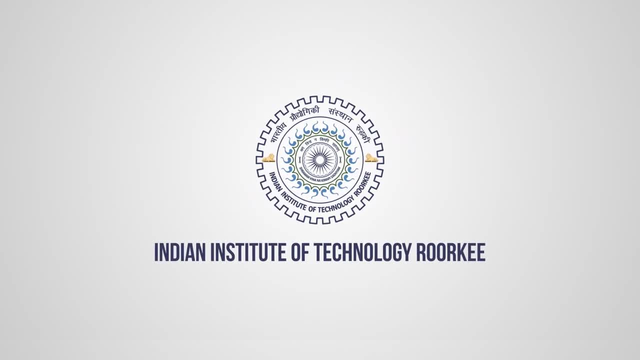 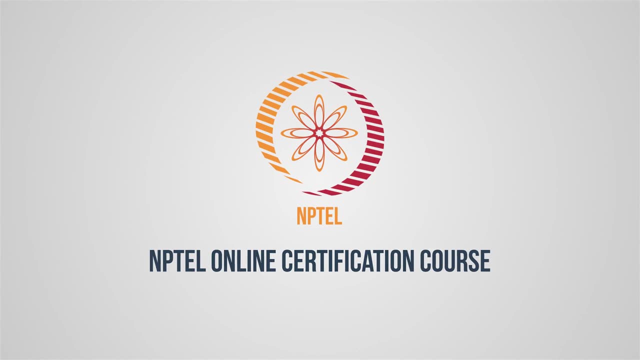 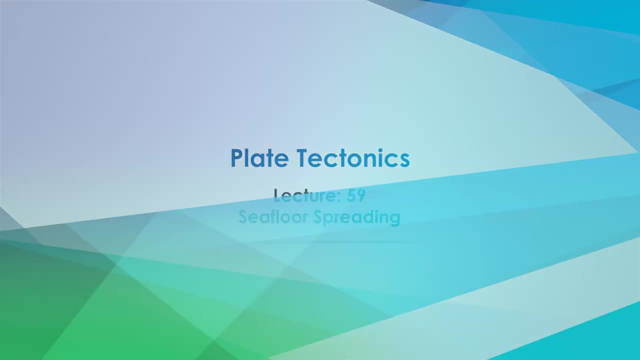 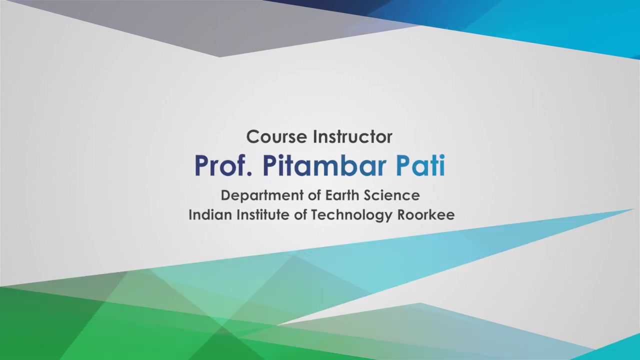 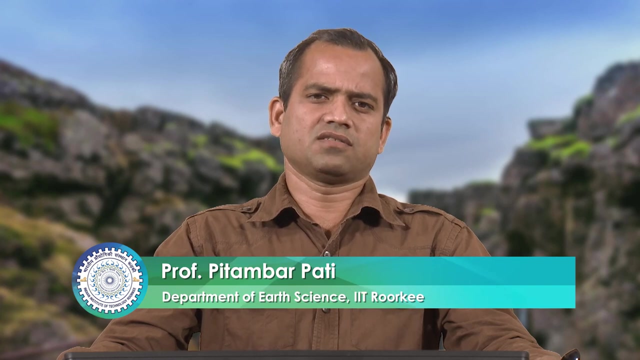 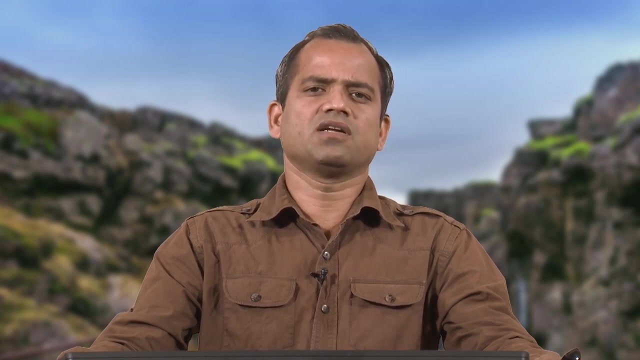 Okay, friends, welcome to this class of plate tectonics. And in today's class we will talk about sea flow spreading. If you remember the last class, we are talking about this continental drift, So that means the continents. once upon a time they were together and with drifting, subsequently drifting, they separated from each other and 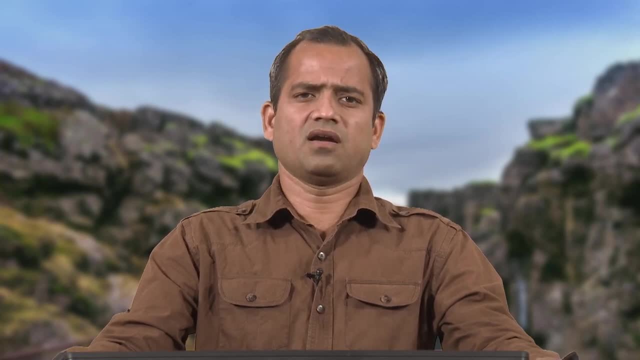 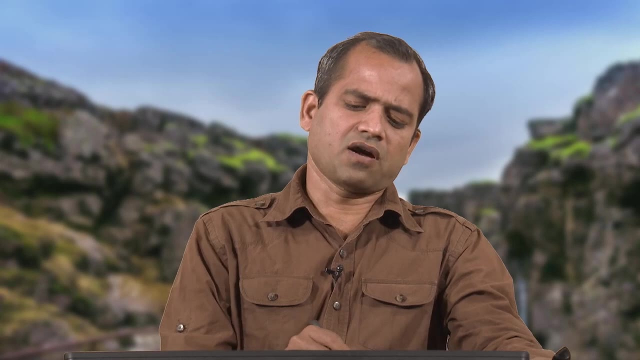 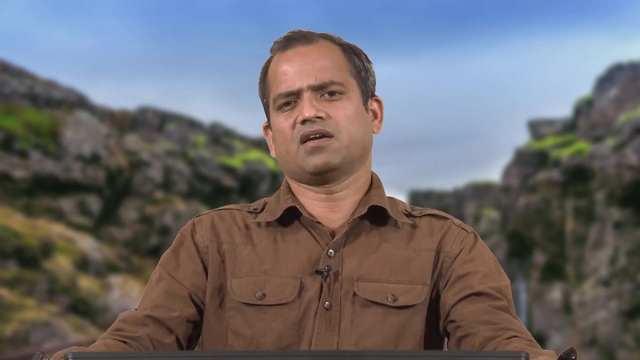 now they are thousands of kilometer apart and separated by ocean floor. So this sea floor spreading, so this is an integral part of plate tectonics and it says about this ocean floor and its characteristics and how this ocean floor is recycled. and what is this? 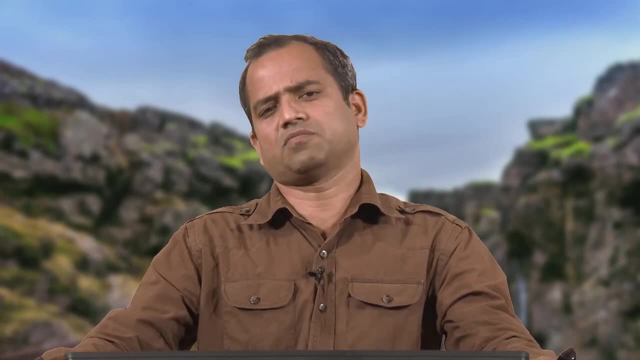 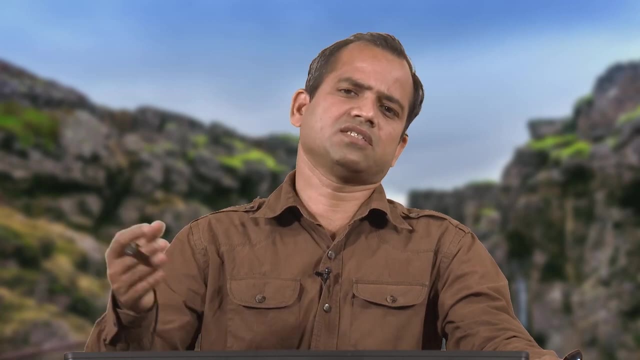 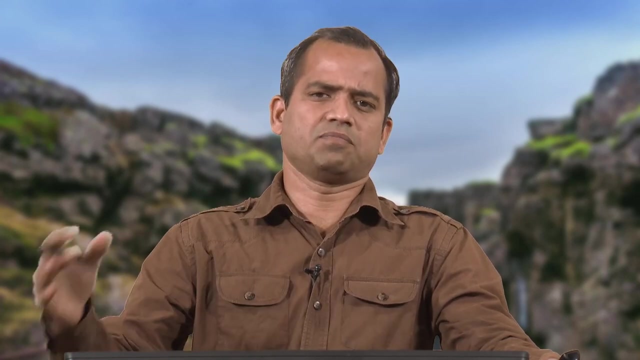 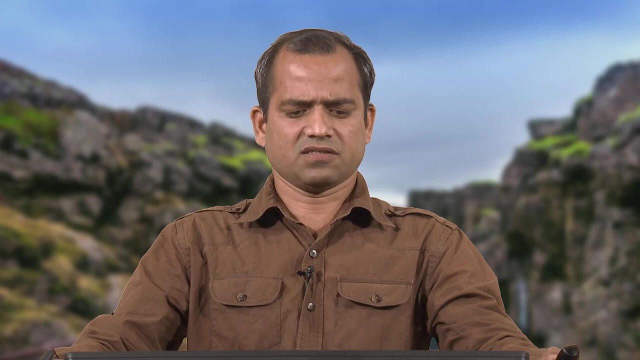 magnetic strips or this magnetic properties of this basaltic carpet that changes with time and its longitudinal change and lateral change. that has been discussed. So, once we know that these continents are drifting, so whether these oceans are spreading or they are constant, that has been discussed in this class. 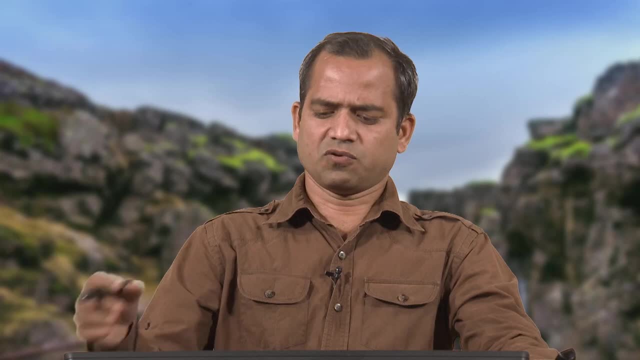 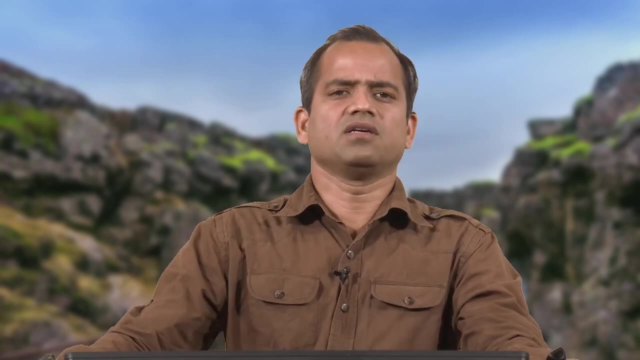 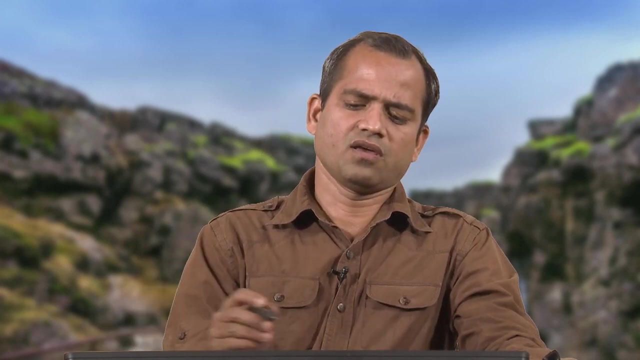 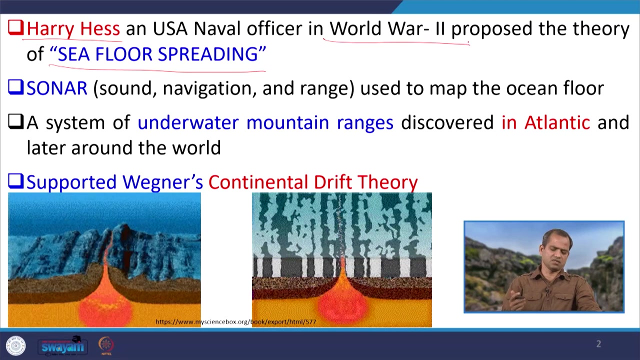 So, like this continental drift, it was proposed by Alfred Wegener, This gentleman, Harry Hess, he was an officer of US Navy, He proposed this sea floor spreading theory and during World War II he proposed this and that he says that, yes, the sea floors are spreading and there are. 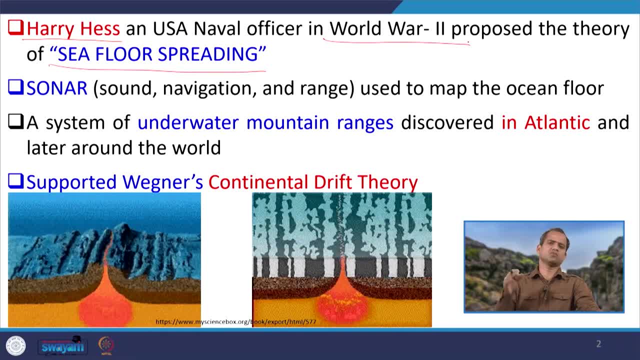 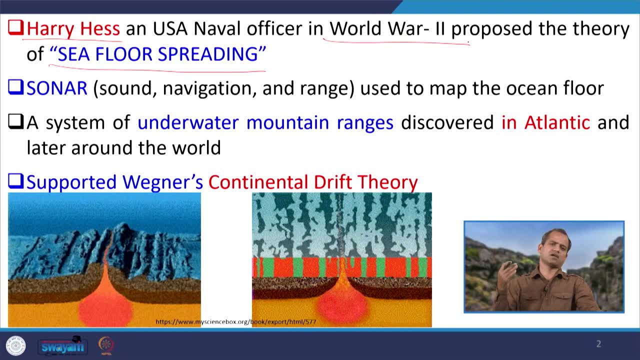 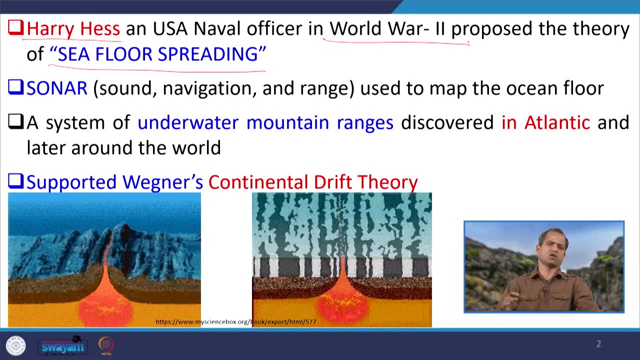 huge mountain chains that is submerged under this oceanic water. So after this World War II, this first this Atlantic Ocean was studied about its subsurface, or about its surface, you can say below the water, and we found that huge mountain chains are there. So after this, 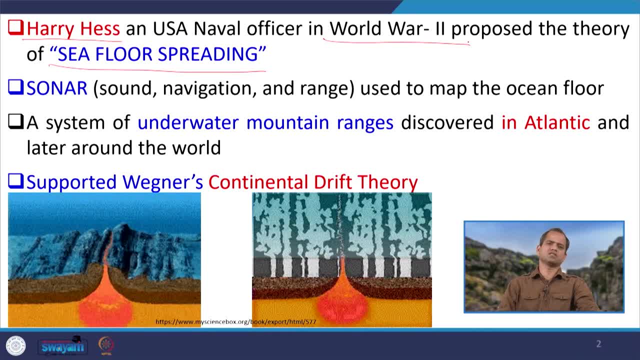 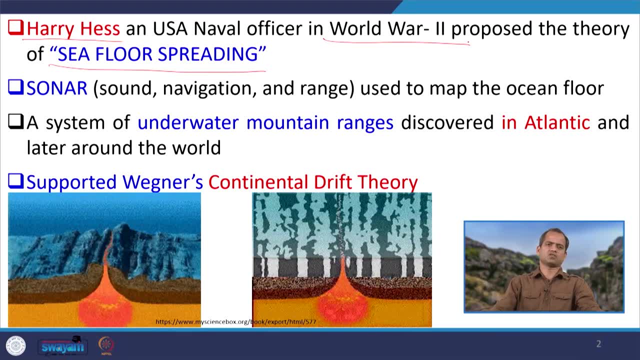 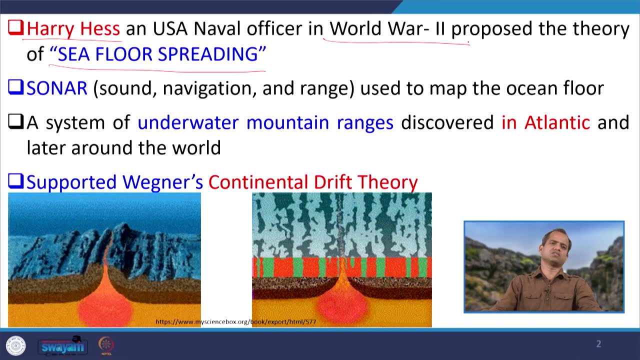 World War II. this first, this Atlantic Ocean was studied about its subsurface or about its surface mountain chain- it is existing- which is submerged underwater, and later on the other ocean floor was studied and similar result was found. yes, there was mountain chains or long range mountain chains there below this water and sea floor. spreading is occurring. 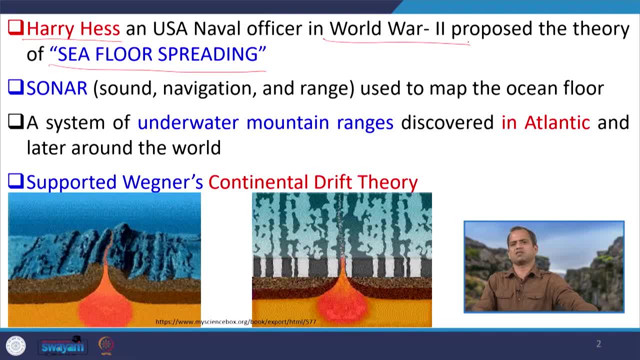 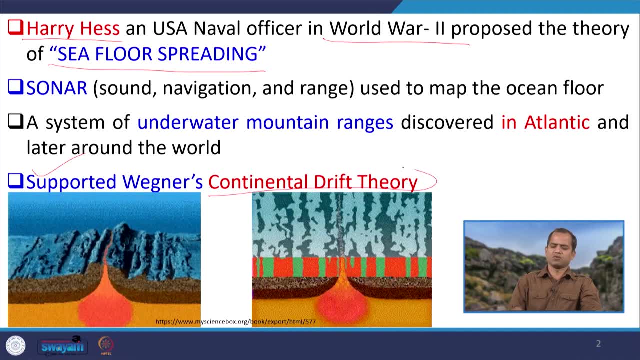 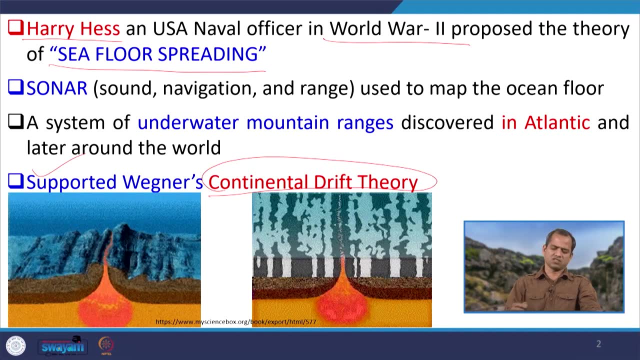 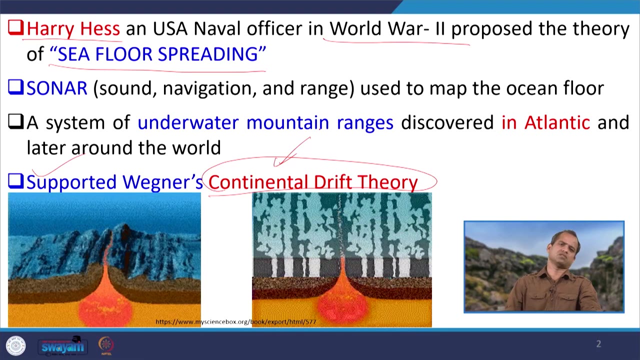 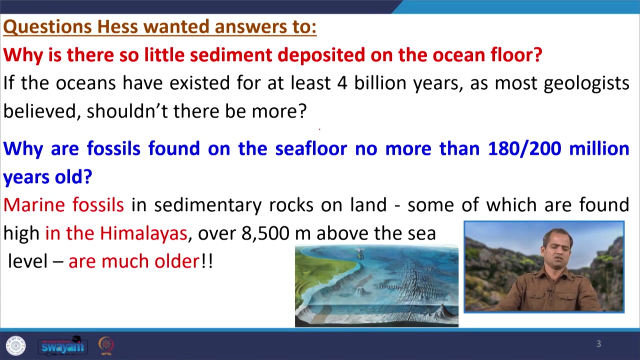 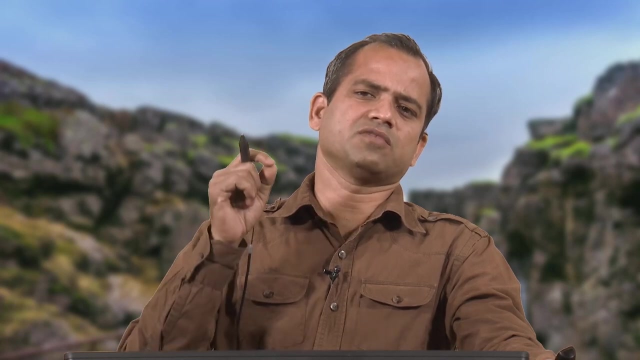 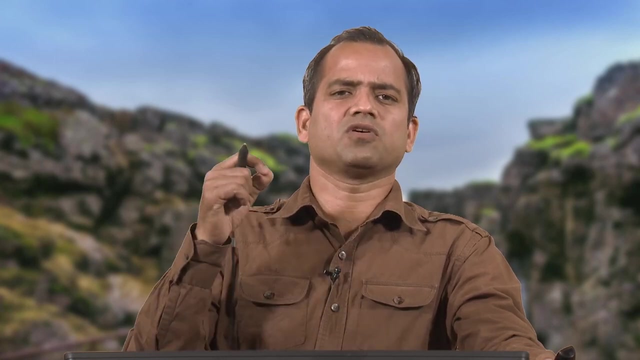 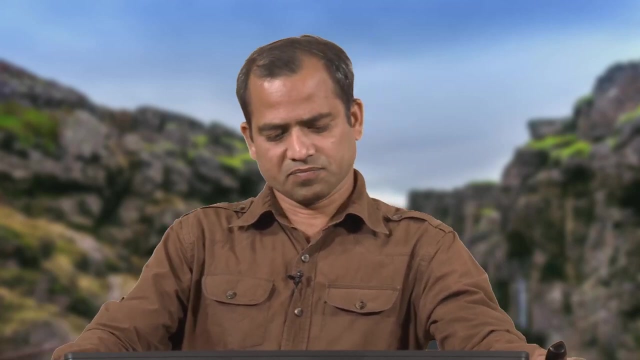 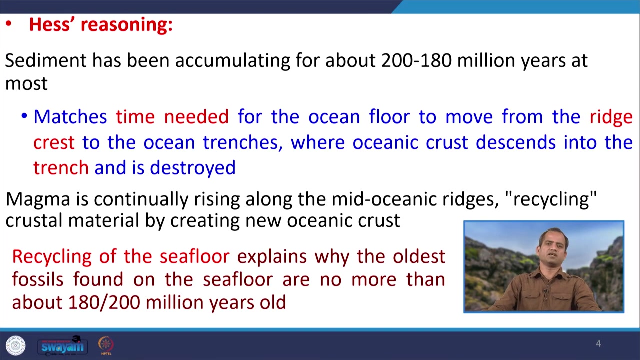 along this. mountain chains, or you can say this: mountain chains are the product of sea floor spreading. This is accumulating for the last 200 to 180 million years at most and this time frame it is matching perfectly. or from this formation of this ocean floor at the mid-ocean creeds. 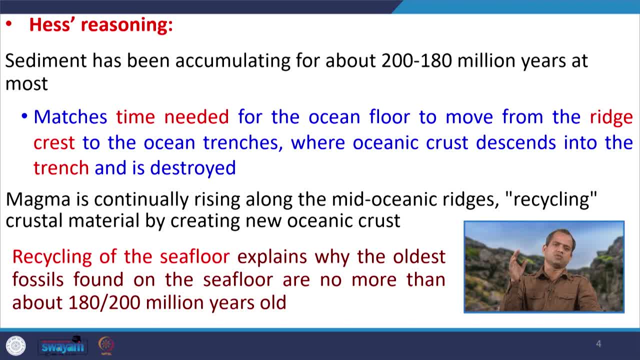 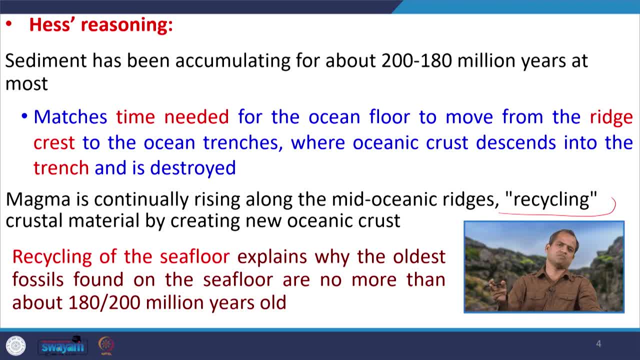 destructive plate boundary where this ocean floor, which is created at a mid oceanic ridge, it is subducting down. So that means you can say, a carpet of basalt which is moving from the mid oceanic ridge and simply it is going down. So this is a recycling process. again it is arising here. 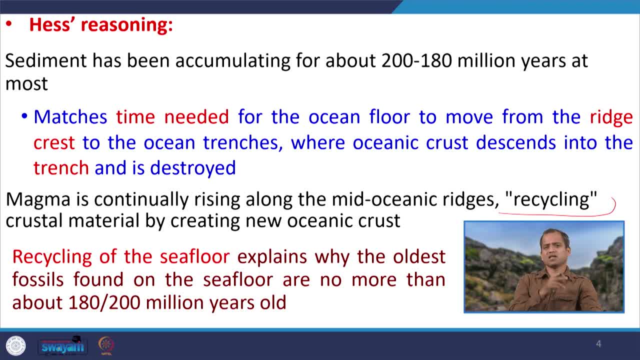 So this is the conveyor belt type, which is recycling this ocean floor system and recycling of this ocean floor. it explains why the oldest fossil found on the sea floor are not more than 180 to 200 million years. So this is the key point to understand. this is the time frame. beyond that, no ocean floor. 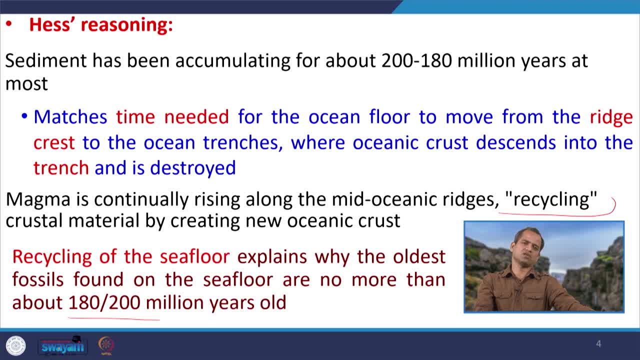 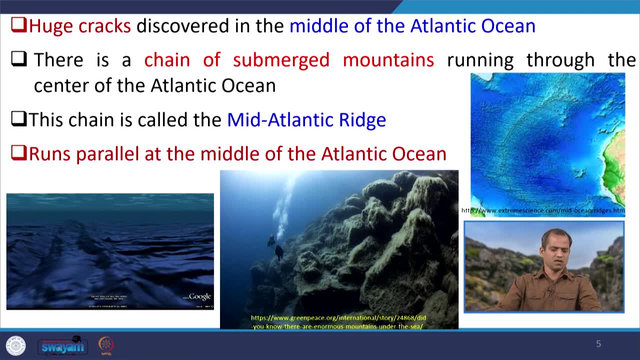 existing live at present day. So that is why, even if the sediments are deposited 400 billion years back, but if the basin is not existing, how can we expect this sediment should be preserved? So some fact about this mid oceanic ridge system and this ocean floor: huge cracks discovered. 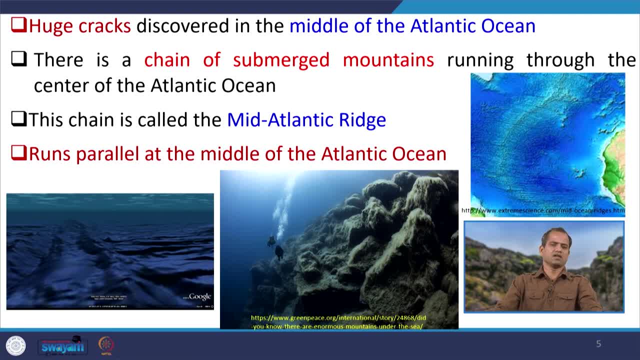 at the mid Atlantic ocean and there is a chain of submerged mountains running through this center of this Atlantic ocean that is called the mid Atlantic ridge and this chain is called the mid Atlantic ridge system and it runs parallel at the middle of this Atlantic ocean. and these are the digital elevation model and this is the underwater photograph. 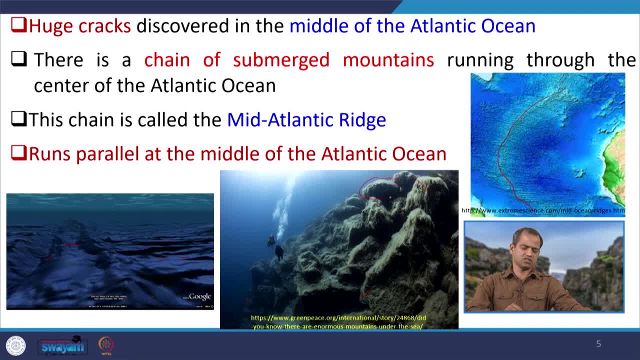 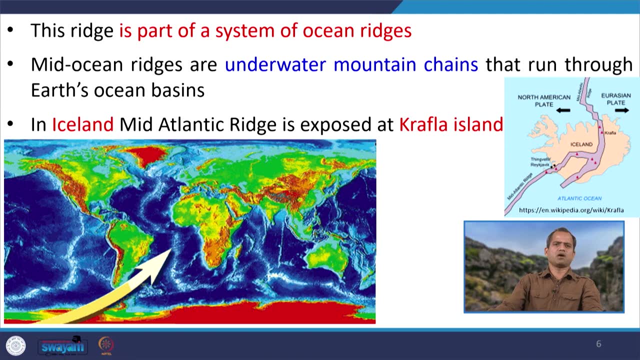 How this mid oceanic ridge looks like the rocks. you can see this pillow basalt. these are the different pillows. they are stacked on one another. So this is the region where this new ocean floor is being created And the ridge is a part of the system of the ocean ridge and this mid oceanic ridges are. 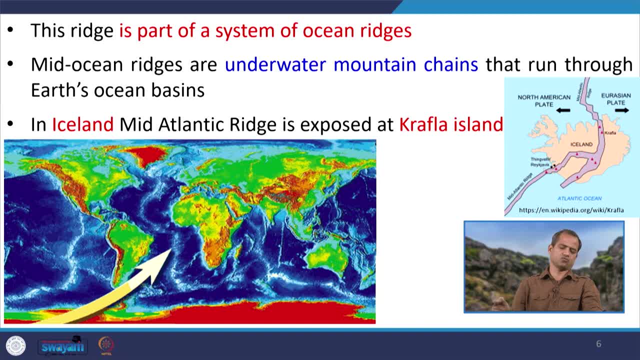 underwater mountains. These are the mountain chains that run through arch ocean basin. In Iceland, the mid Atlantic ridge is exposed at Krafla island, So if you want to see this mid oceanic ridge, it is totally submerged underwater and you can say submerged under deep water. however, at the only place, that is the Krafla island, 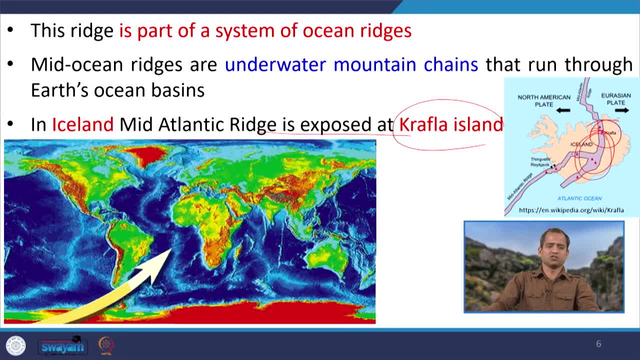 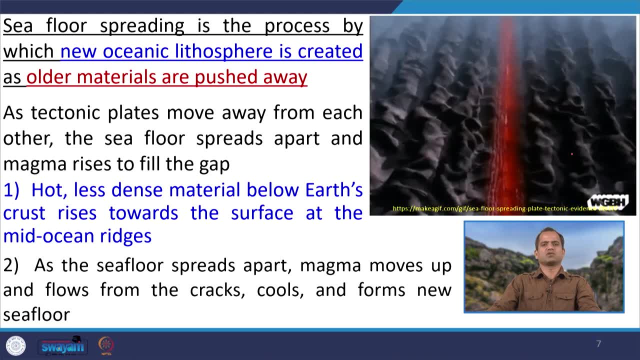 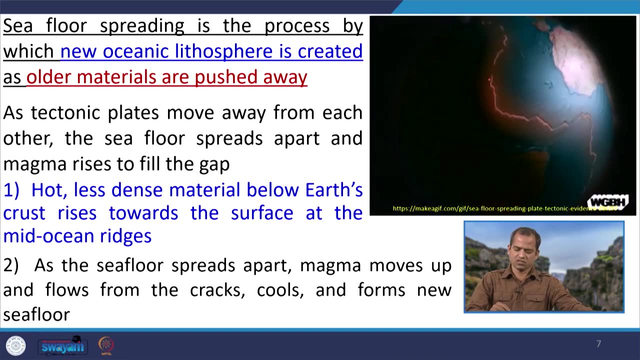 so here the mid oceanic ridge is exposed. you can go for geotourism and the sea floor spreading. it is the process by which new ocean lithosphere is created and the older material are pushed away. So here you can say: this is the ocean floor and you see, if you zoom this ocean floor and 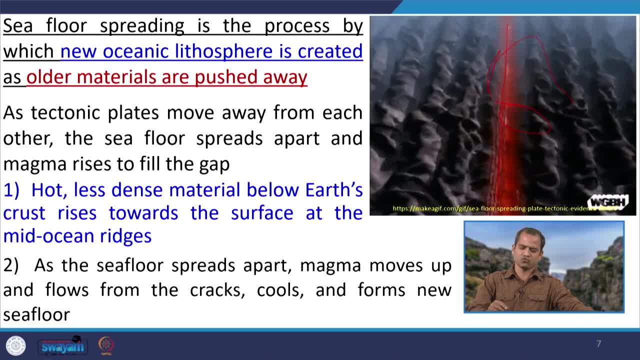 particularly the mid oceanic part, if I am zooming this region. so I am creating this type of image in my mind that here this is a huge crack existing and through this crack the magma is erupting continuously. So this is the crack And the erupted magma, once it is reaching to this subaqueous environment, it is creating. 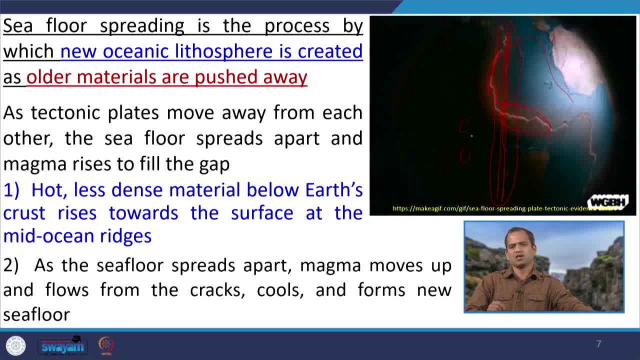 some pillows, that means pillow basalt is developed and this pillow basalt, it is forming a carpet and from here this plot is moving in this direction and this other part is moving to other direction and finally it becomes a part of this solid oceanic crust. 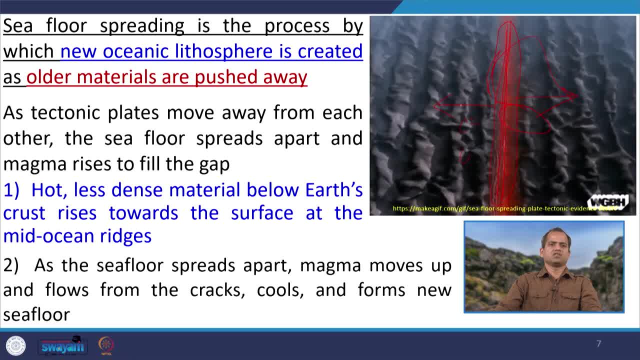 So as the tectonic plates moves away from each other, The sea floor spreads apart and magma rises to fill the gap. So hot and less dense material below the earth's crust rises toward the surface at the mid oceanic ridge system. As the sea floor spreads apart, magma moves up and flow from this cracks and cools and 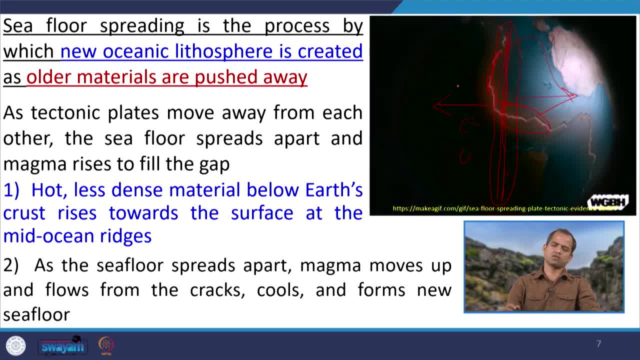 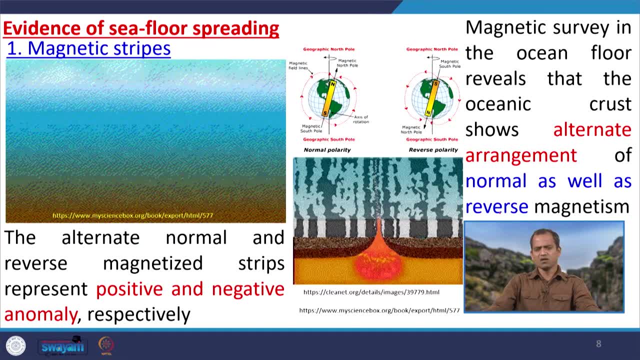 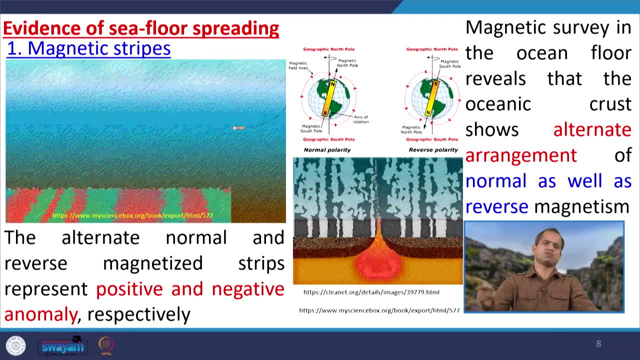 forms new ocean floor. So this ocean floor basalt, or the ocean floor illo basalt, it is a product from the mid oceanic ridge system. Now, whatever the fact we are discussing about, we must have some evidences. Yes, sea floor is spreading because, if you remember, when you are talking about this continental 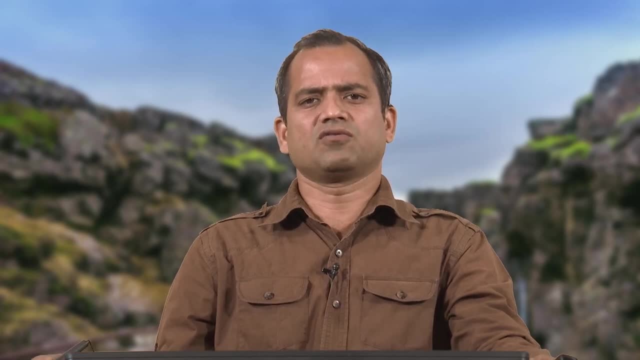 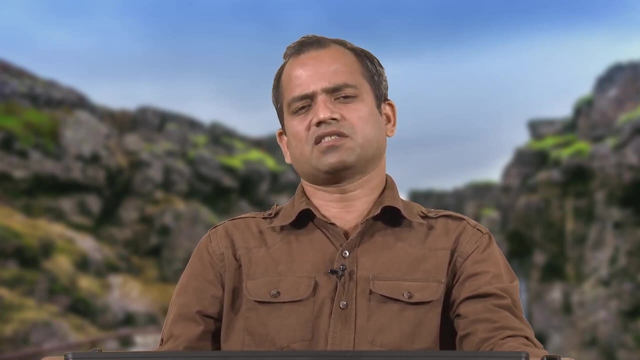 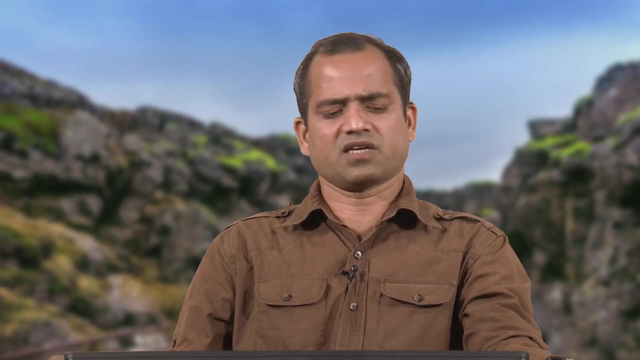 drift. we have to provide number of evidences to prove yes, the continental drift is occurring. Similarly, to provide this, evidences about the sea floor spreading. number of experiments and the number of field observation was carried out. number of studies was carried out and one of these foremost study. 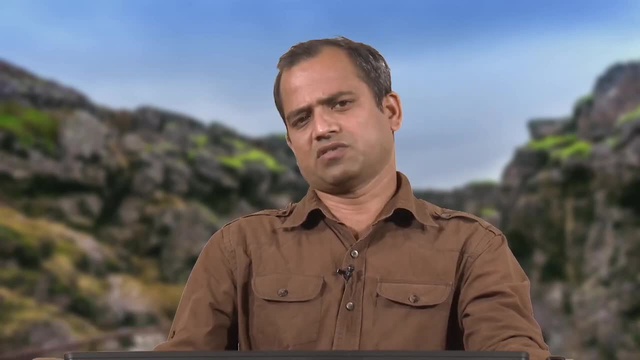 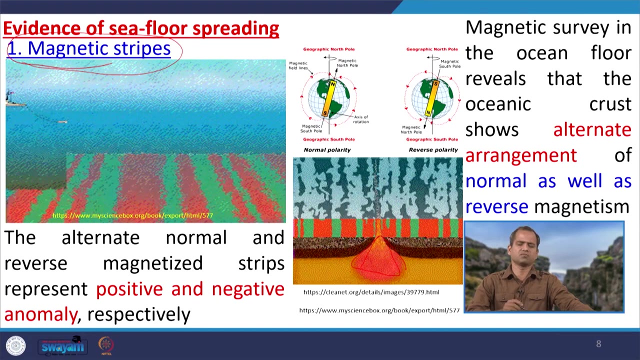 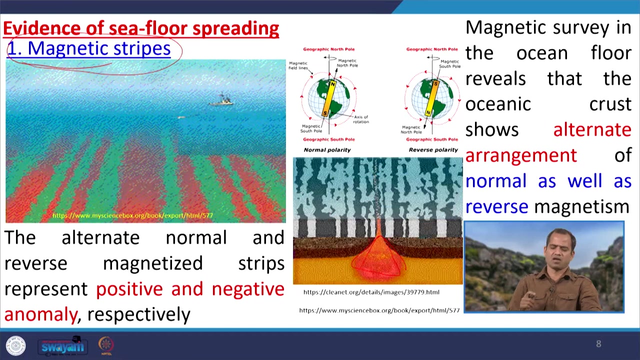 Here is the magnetic strips. Magnetic strips that means, if you see, when we are creating this mediocinic ridge basaltic system at the mediocinic ridge, this basalt having some minerals, ferromagnetian minerals, and those ferromagnetian minerals, they are aligning themselves and with the 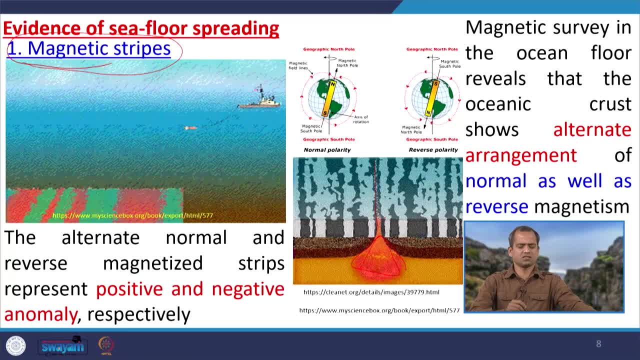 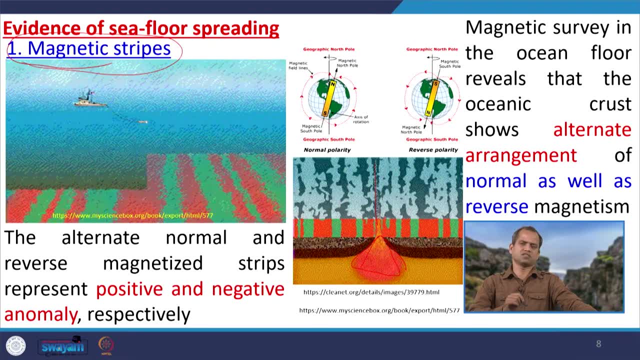 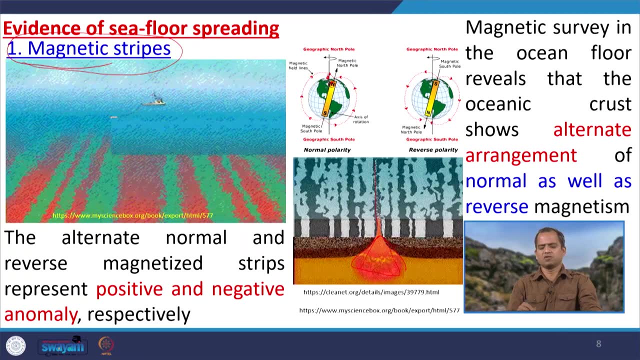 existing magnetic field and we know this earth is magnetic field which is reversing and with geological time and the rate of reversal is not same throughout. For example, here this is the geographic north pole and this is the magnetic north pole. if the geographic north pole and magnetic north pole, they are in the same hemisphere, we say 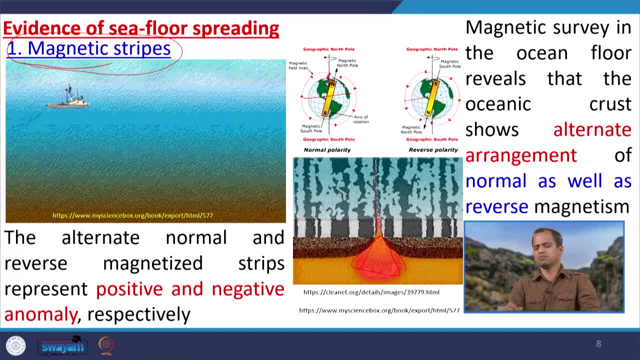 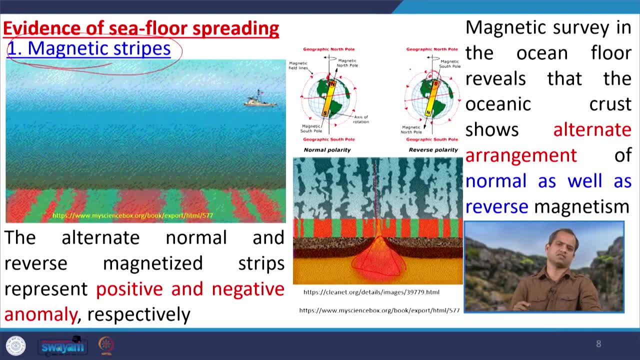 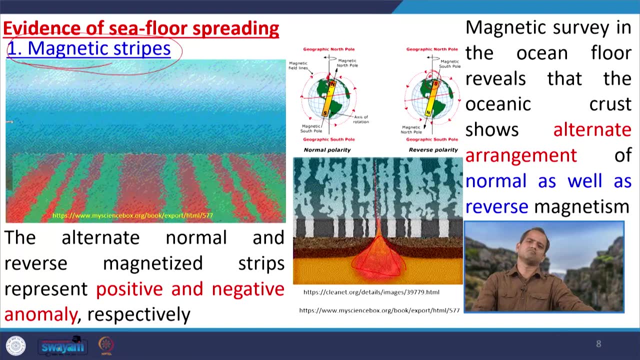 it is normal magnetism. But if the reverse is true, that means we have geographic north pole and magnetic south pole In the same hemisphere. that is called reverse magnetization. So that means these reverse and normal magnetization. it happens in earth history and in geological past, in stratigraphic. 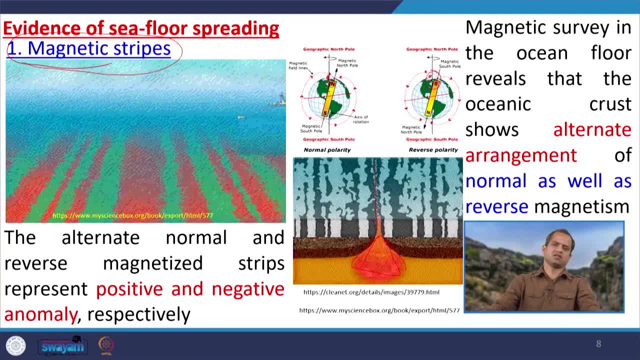 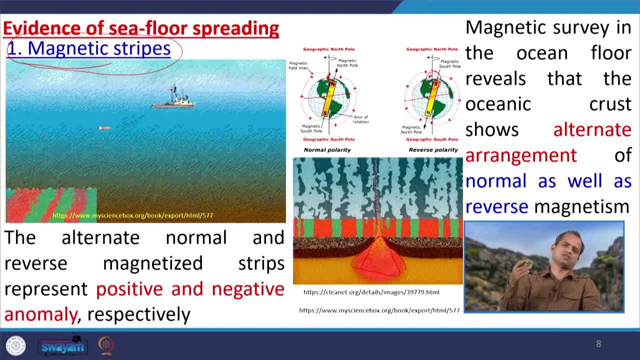 record. you will see number of times the earth has recorded the normal magnetization and reverse magnetization And the duration is not constant. you cannot say there is a continuous. duration is there, So that means it may be millions of years. there will be prominent normal magnetization. 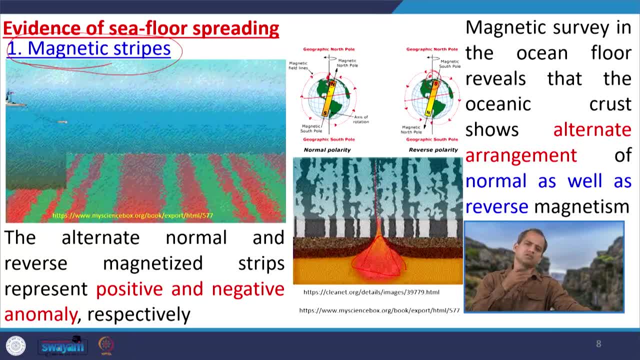 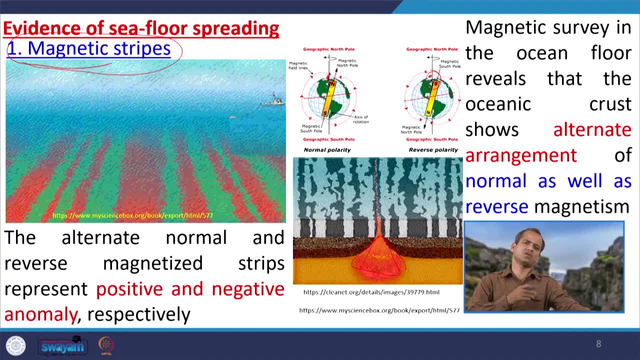 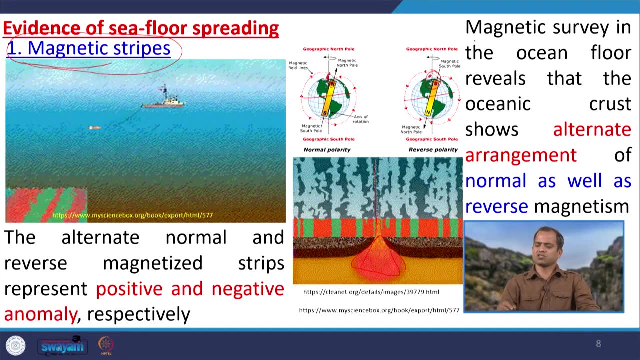 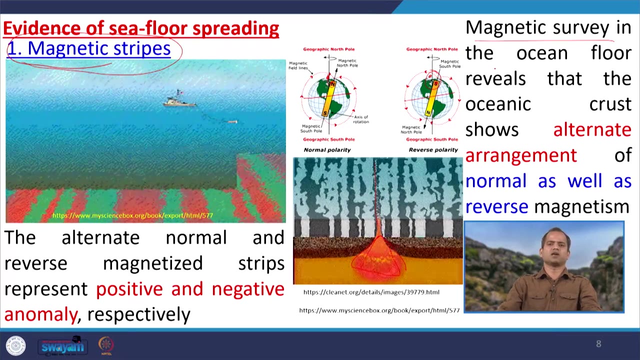 And reverse magnetization also prevailing for millions of years and it may have changed in thousands of years. So that means there is no constant way and it is not properly understood yet why it is happening. so So that means, if you see, this magnetic survey in this ocean floor reveals that the oceanic crust shows alternate arrangement of normal. 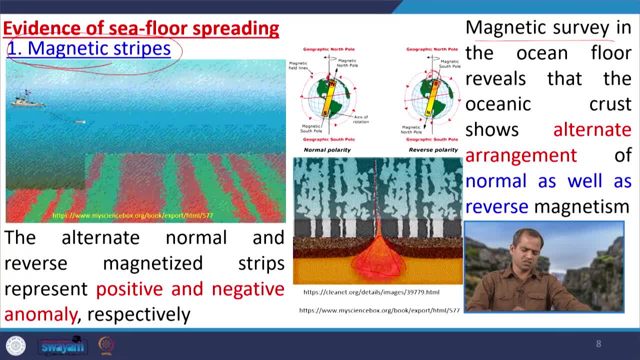 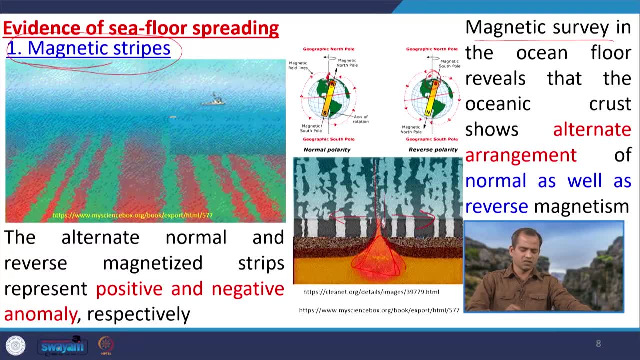 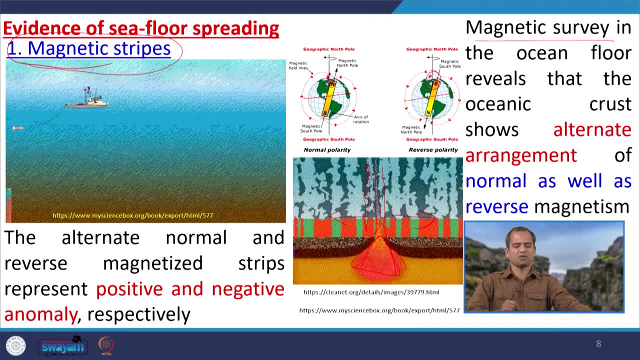 as well as reverse magnetism. So you can see when this basalt is forming here and is two plates are moving away from each other, whenever, suppose, for example, here this black color. So here that means this black color is forming. that means suppose, for example, it is normal. 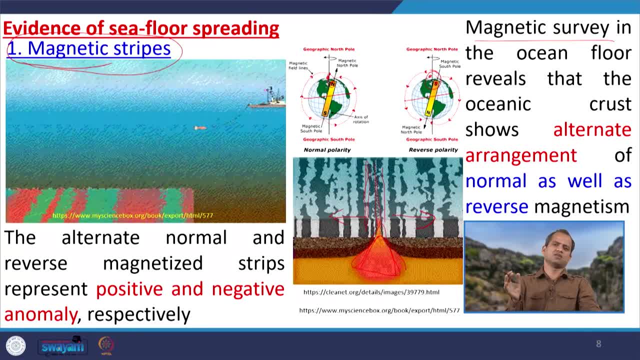 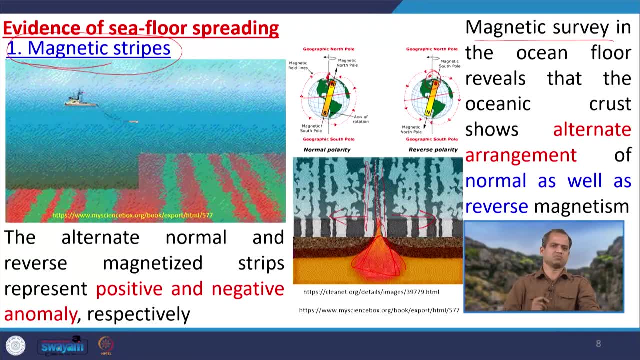 magnetization. And here that means at this stage this earth magnetism is normal stage. So that means geographic north pole and this magnetic north pole. they are in same hemisphere. So that means, if it is happening, so whenever these rocks are forming, so there magnetic. 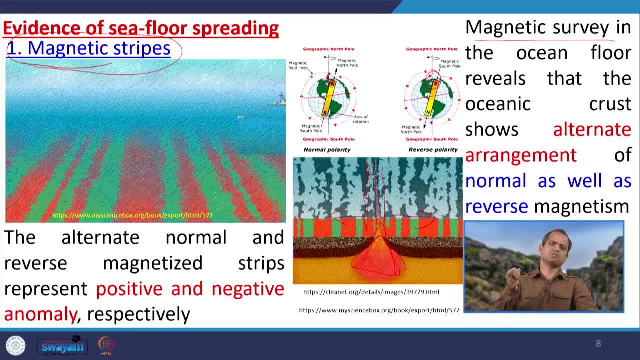 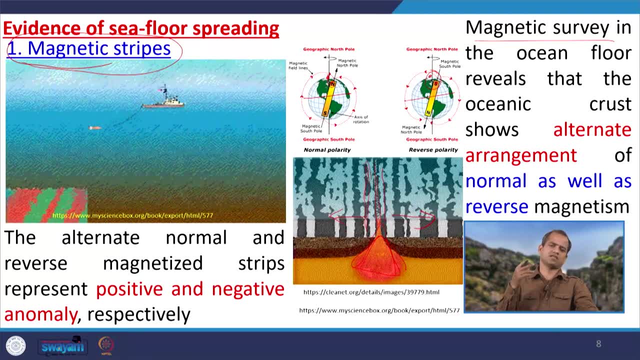 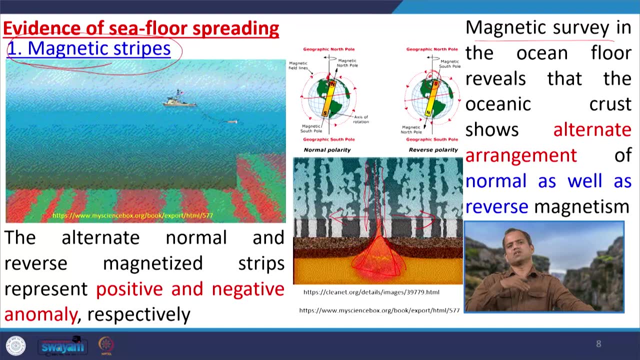 minerals they are aligning with respect to that And after suppose for thousands of years it changes. that means reverse magnetization occurs. So the rock which will form at that time, that will record that reverse magnetization within their magnetic minerals. So that means that is why with the change of magnetic reversal and normal system, the 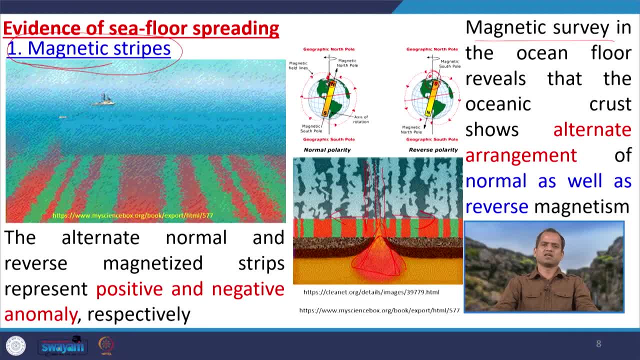 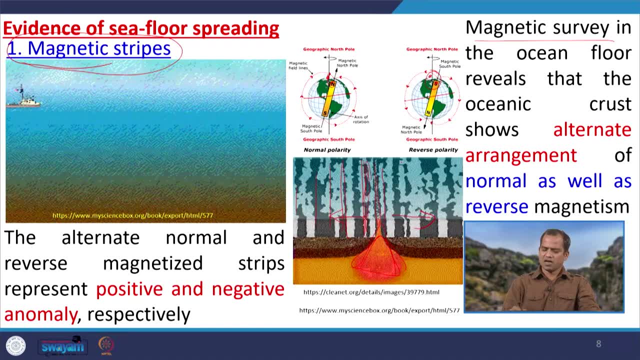 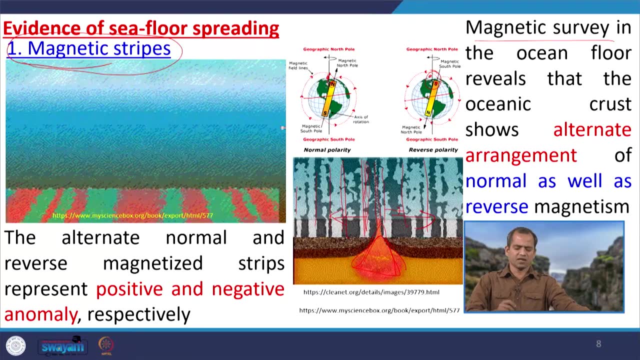 rocks which are forming from the meteosinic ridge. they are aligning and they are forming the strips which is corresponding to this existing normal and reverse magnetization duration And the width of this strip. that depends upon two factor. One factor is the rate of motion and another factor is the duration of the normal and reverse. 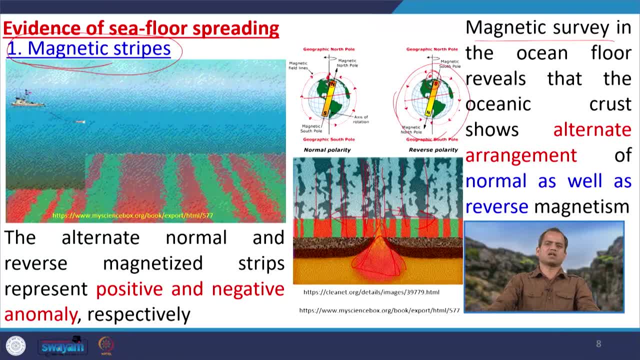 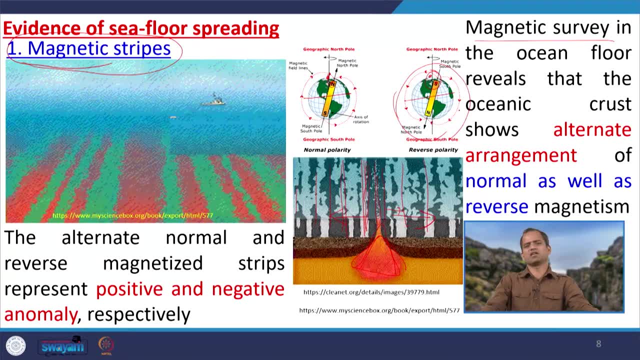 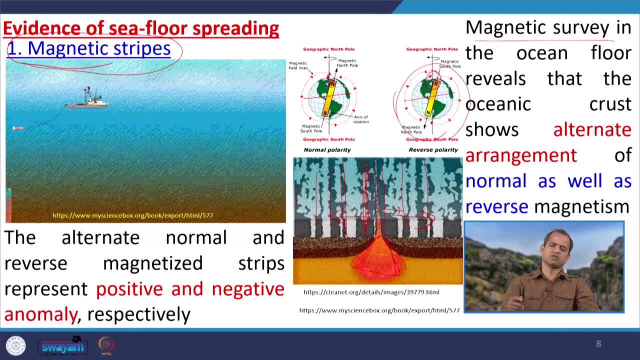 magnetization If, for a longer geological time, normal or reverse magnetization occur, so this strip width will be more. Similarly, if the rate of spreading is more, a strip width will be more. So depending upon this strip width, you can say whether this rate of spreading was more. 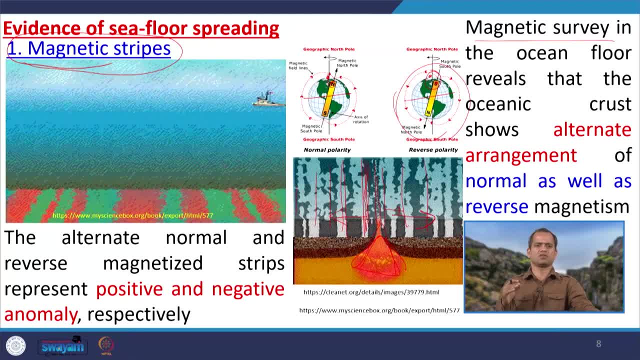 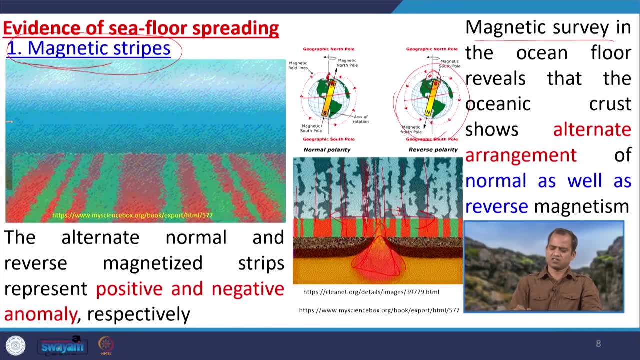 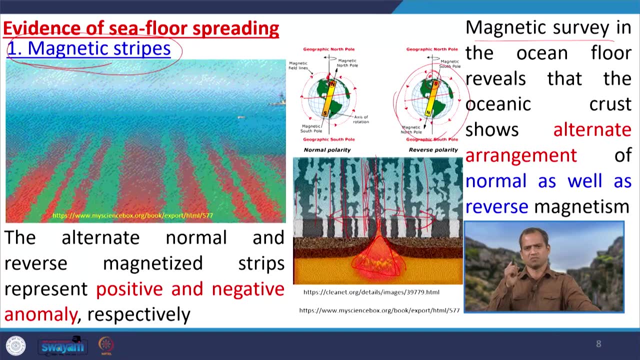 or this duration of this normal and reverse magnetization work for a more time. So now we have a alternative strips of normal and reverse magnetization that is occurring from this meteosinic ridge system and it is embedded within the basaltic rocks, within that magnetic minerals. 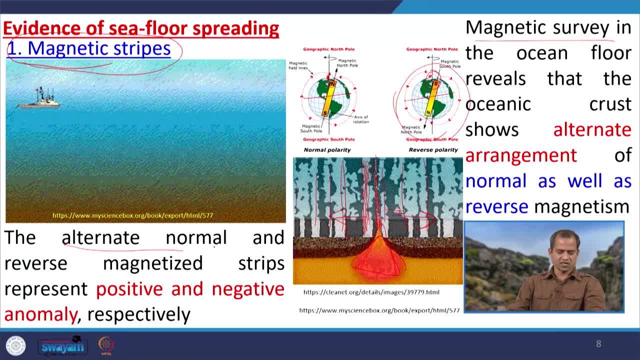 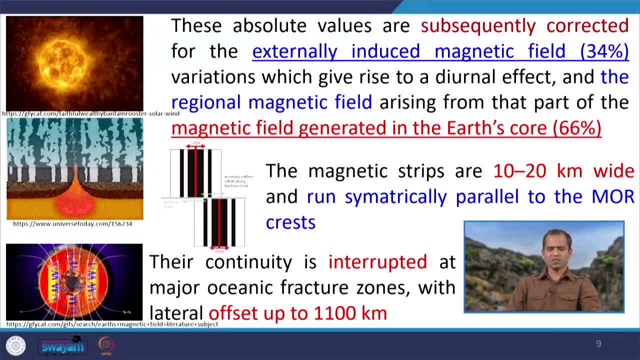 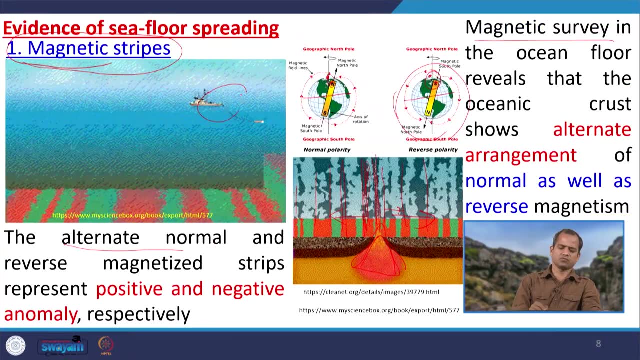 And the alternate, normal and reverse magnetized strips represent four factors, And positive and negative respectively. that already we have discussed. Now the question arises when we are having this magnetometer. it is attached with the ship. you see, this ship is moving and this is the magnetometer. 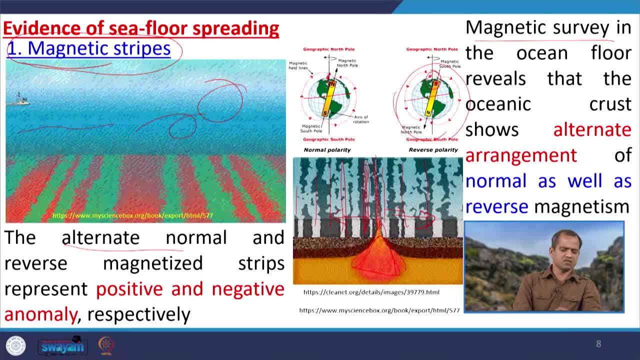 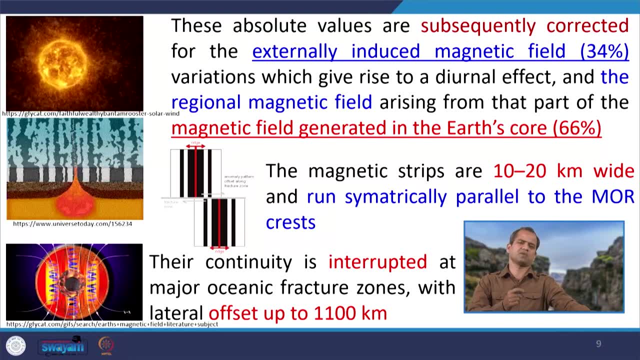 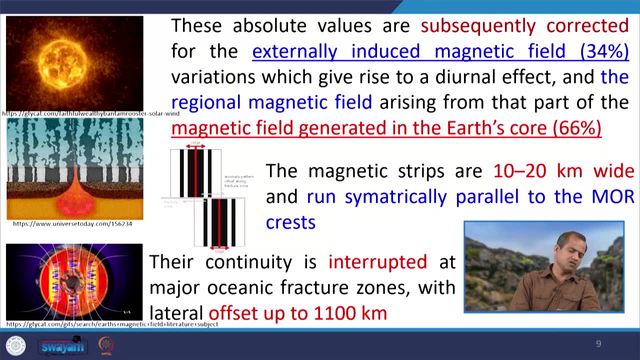 So this magnetometer, once it is moving, and it is recording this normal and reverse magnetization as a strips. So this rock magnetism which is recorded by this magnetometer, it is affected by two factors. One is the internal factor. that means that is the convection current at the outer core. 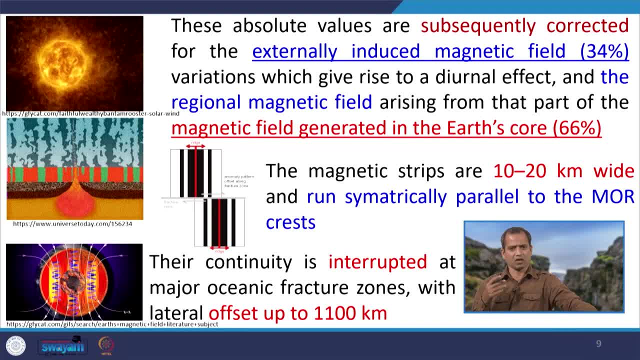 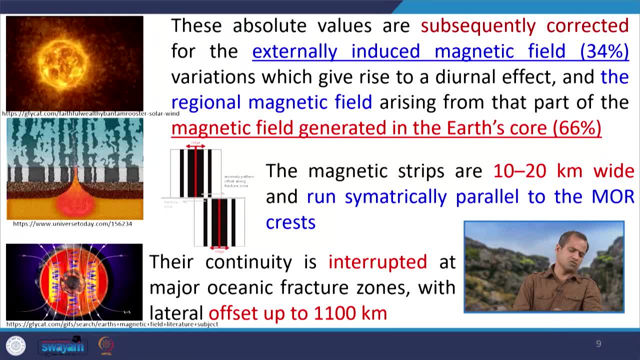 and we know in your initial classes. when we are talking about this earth's internal structure, when we are talking about this outer core configuration, we are talking that this outer core, due to this movement of this magnetic materials there will. it is working as a dynamo and a electric field and subsequent the magnetic field is generated and that magnetic field 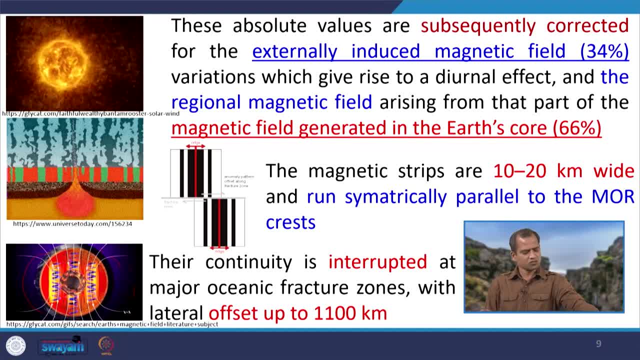 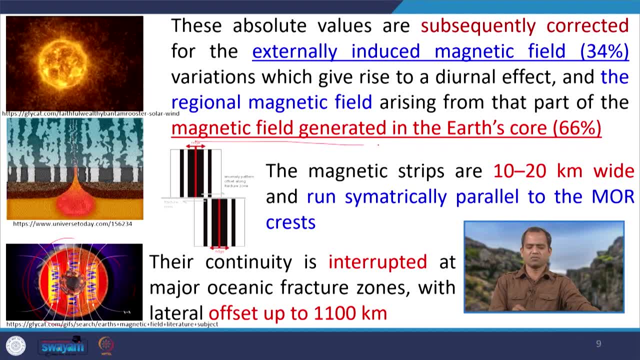 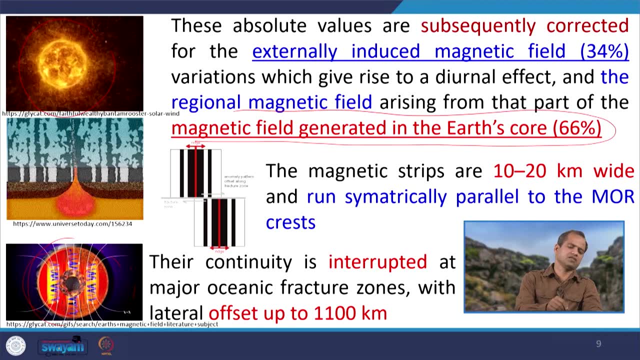 it is affecting to the surface- magnetization. Ok, So that is called the internal system. So one contribution to the rock. it is by this earth's internal field, generated from this earth core. another system which is affecting the rock is from this external field. that 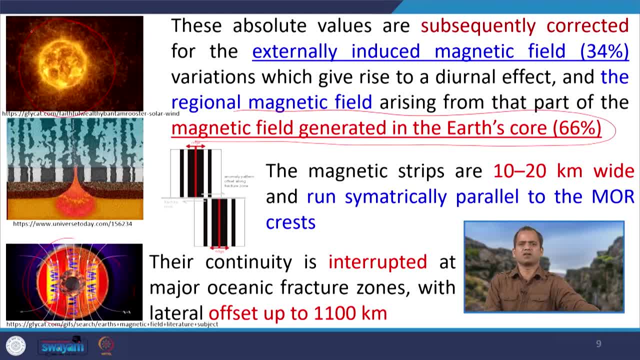 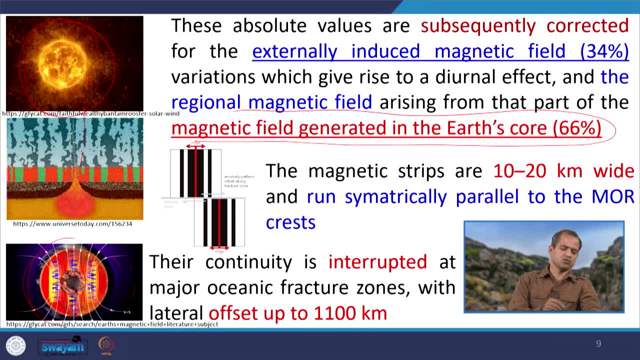 is from the sun. We have solar wind, we have different magnetic storms and due to this magnetic storms- the solar wind- it is also affecting our rock here, So that means a rock which is crystallizing on the surface of this rock. It is affected by this external factor and also affected by the internal factor. 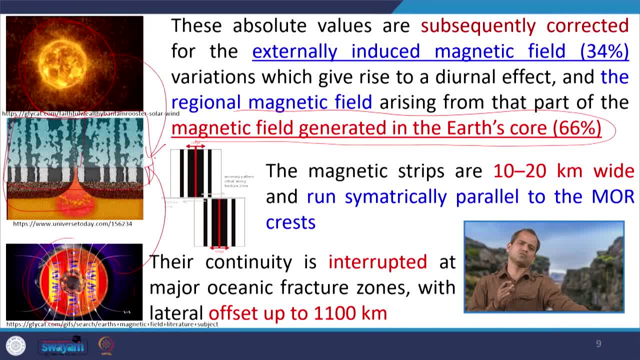 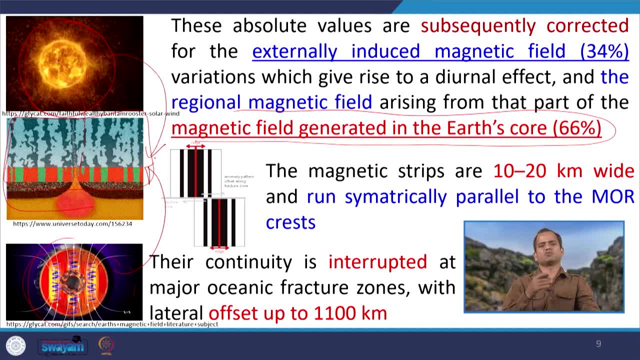 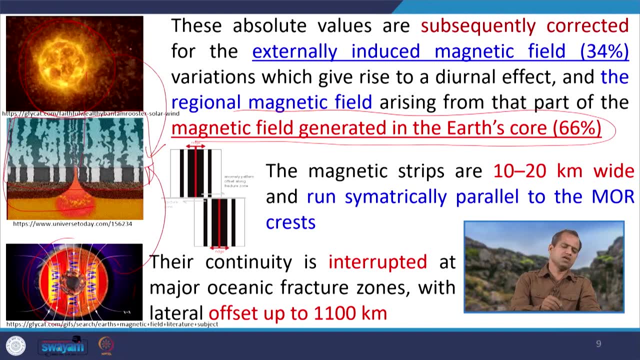 Now the question arises: as a geologist, our aim is to know about this internal system, to restrict our self to this internal contribution of magnetization, because we are interested to construct the magnetic poles. So that is why we have to clean, we have to rule out this external influence. that is why 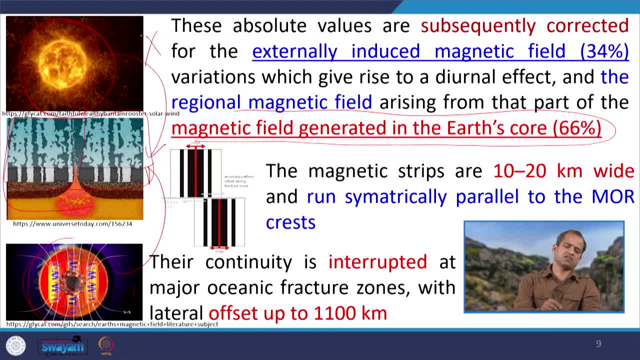 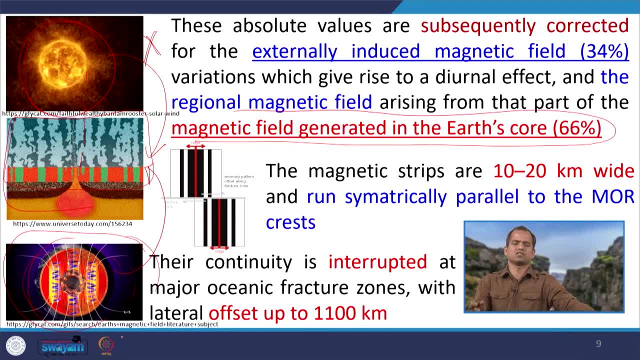 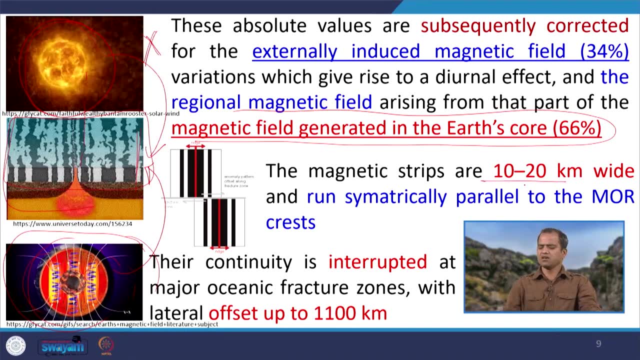 we go for ignoring or cleaning of this external influence from this total one. So the remaining one is the internal influence, that is, from this convection system at the outer core system And those magnetic strips finally we are getting. they are 10 to 20 kilometer width and run. 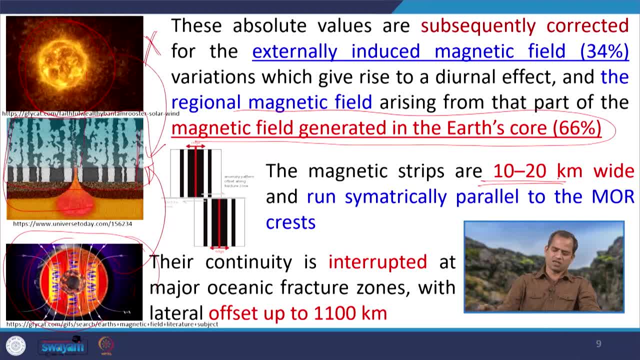 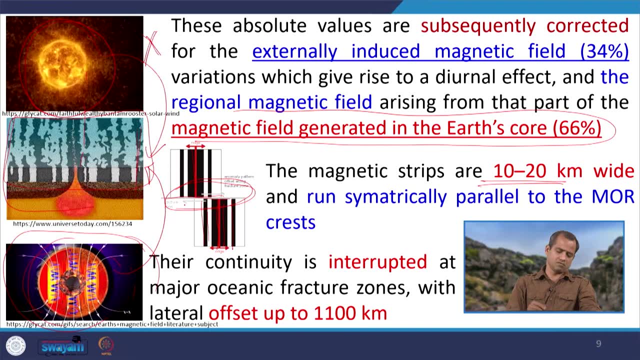 symmetrically parallel to the mediocentric system and their continuity. it is just hindered by this transmission. For example, here you see, this is the mediocentric system and these are the strips of normal and reverse magnetization. and had it been not here, that is, the transform fault is not. 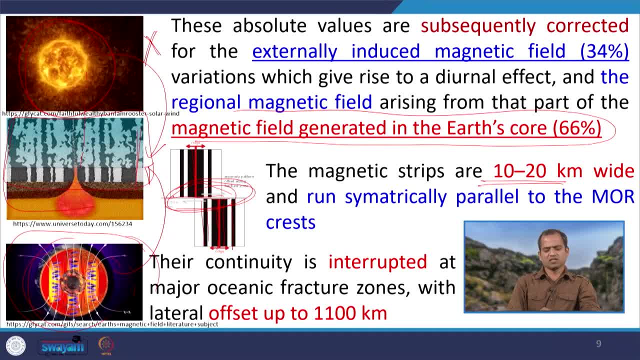 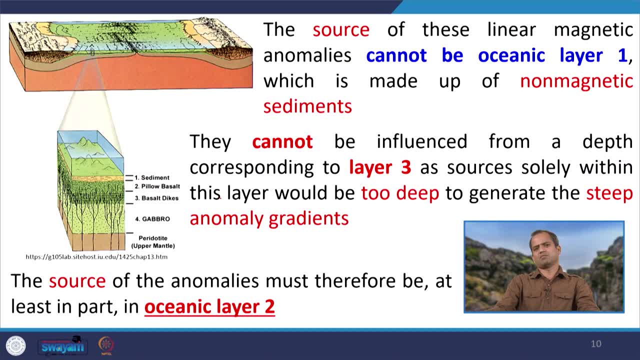 there, that will be continuous. So that means this continuity. it is broken by this transform fault. here Now the question arises if we are having a magnetometer which is attached to the ship and it is moving on this ocean water And it is recording the magnetic field. 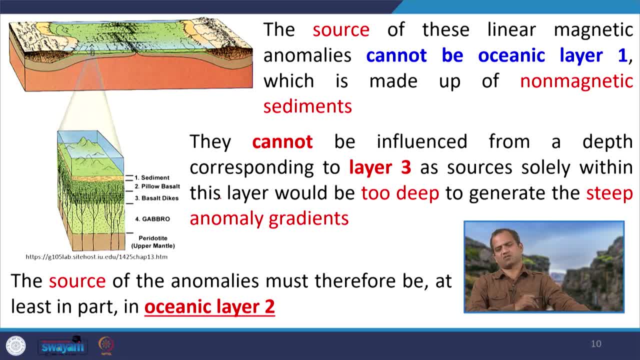 So which layer of this oceanic crust or which layer of the oceanic lithosphere it is contributing to this magnetometer. that means the rock magnetization is contributed to the magnetometer Because if you see this oceanic lithosphere, when we are talking about the initial class, 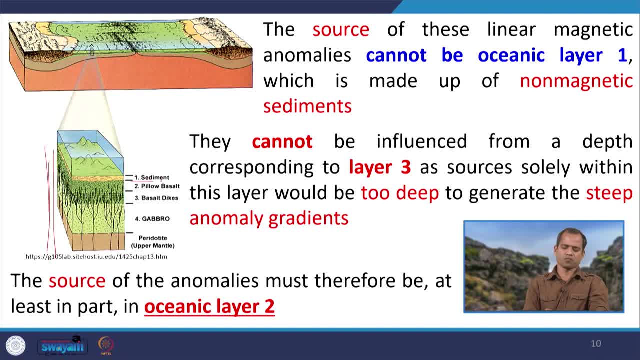 about the oceanic lithospheric composition. We have layer 1, which is sediment mostly. it is not ferromagnetism, it is quartz of feldspathic sediment. So that means this layer 1, as it is not suitable composition, that means magnetically suitable. 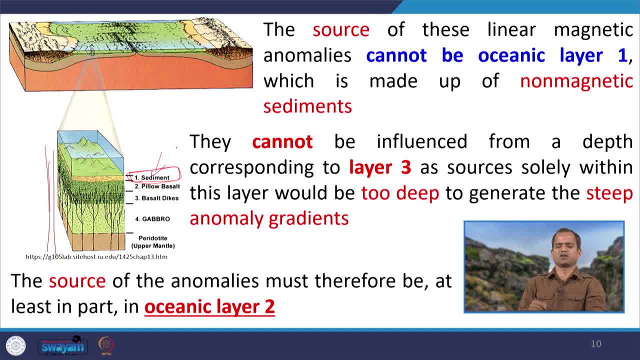 composition. So that is, its contribution to this magnetometer is negligible, So we ruled out. Now come to this layer 2, which is of basaltic origin, and it is enough magnetic mineral is there that can influence. and third is the layer 3, that is the gabbro and which is the 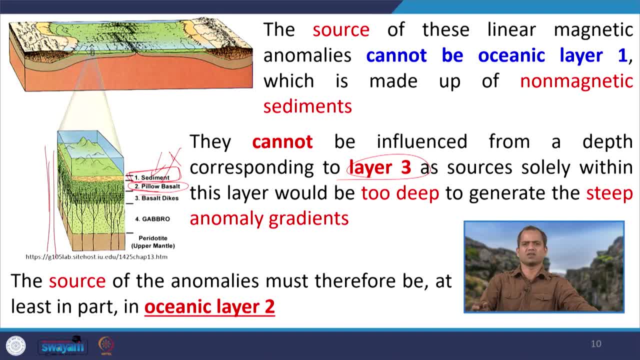 pylori, though it is containing magnetic mineral. gabbro pyridotite: it is containing magnetic mineral, But as their depth is too high, their influence to this magnetometer, which is near to the surface water surface, is negligible. So that means layer 1 we ruled out because it is composition. 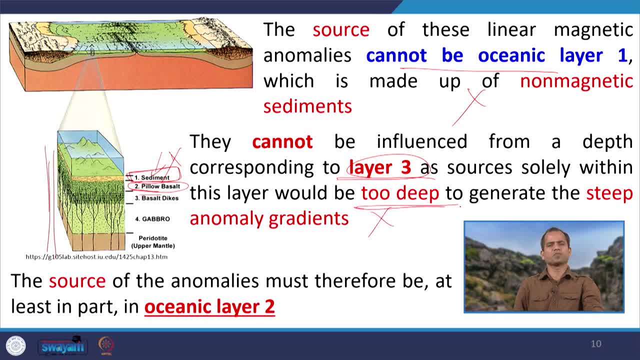 Layer 3 we ruled out because it is too deep. So the next one is the oceanic layer 2.. That is the pylori layer. So the next one is the oceanic layer 2.. That is the pylori layer. So that means the pylori basaltic layer, which is the main contributor. 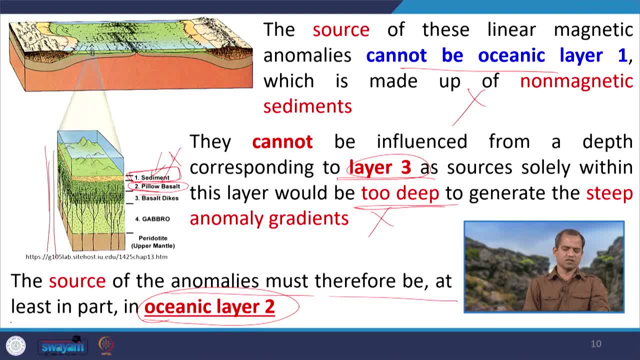 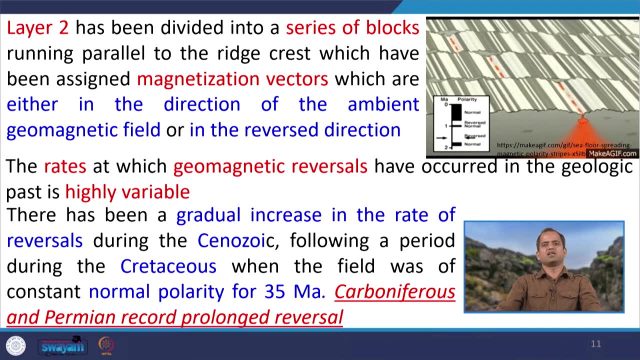 So the source of anomalies must be therefore, at least at part, by the oceanic layer 2.. So that means the pylori basaltic layer, which is contributing to the magnetometer to study the magnetic strips, and layer 2 has been divided into a series of blocks running parallel to. 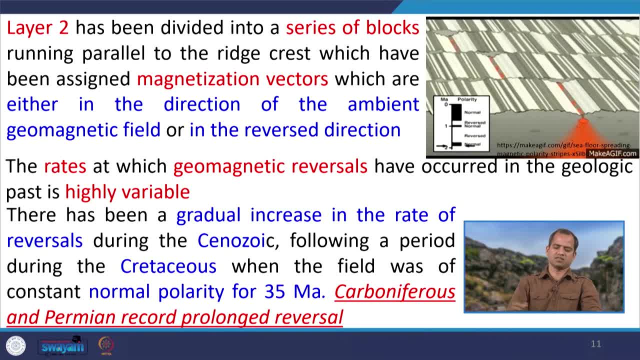 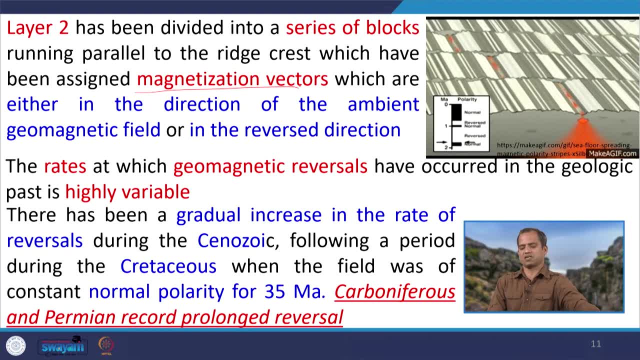 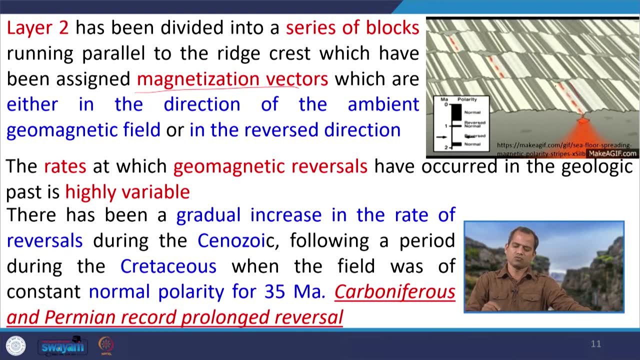 this ridge crest, which have been assigned magnetization vector And which are either in the direction of ambient magnetic field or in reverse direction. So that means this normal and reverse magnetization, if you can see this animated image. So we have reverse and normal magnetization and you see how this with time, when there 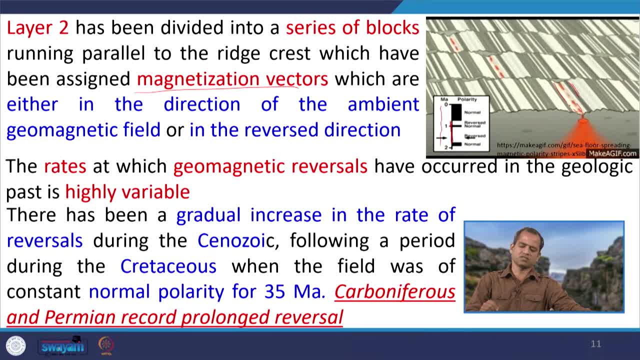 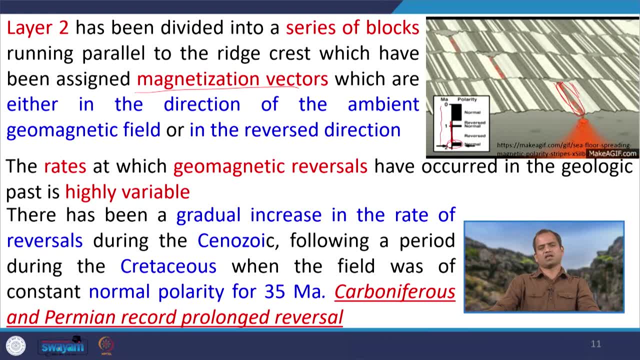 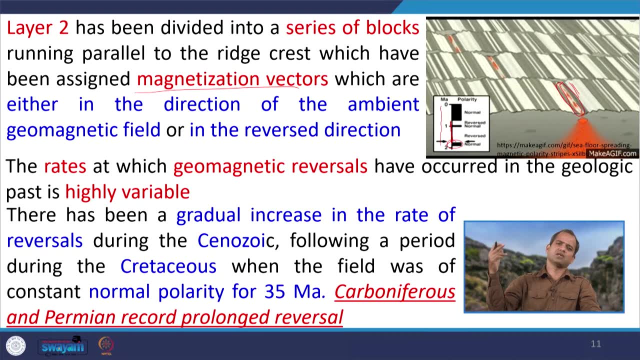 is a normal period, whatever the rocks are forming, that is also recording the normal magnetization. When it is reverse period, when this rocks are forming, they are recording the reverse magnetization. So this normal reverse, normal reverse, that depends upon the earth's magnetic field existing. 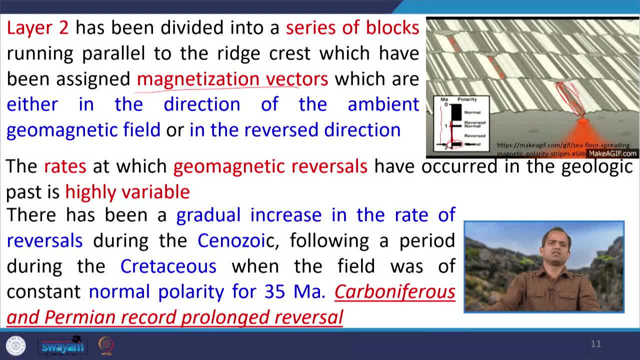 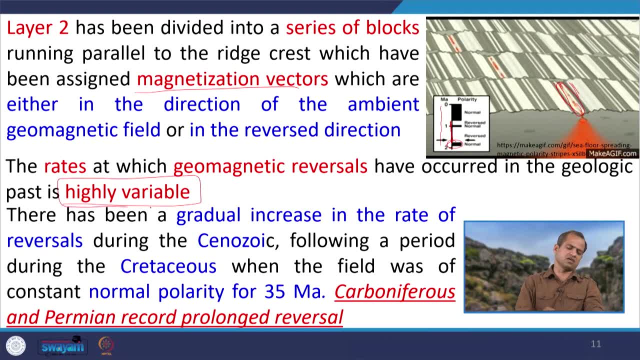 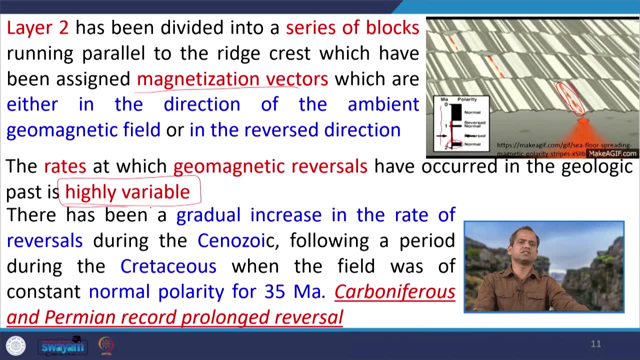 that time and the rate at which the geomagnetic reversal that occurred in geological time it is highly variable. No constant duration is there that this earth's magnetic field will change and there has been a gradual increase in the rate of reversal during synozoic period following a period. 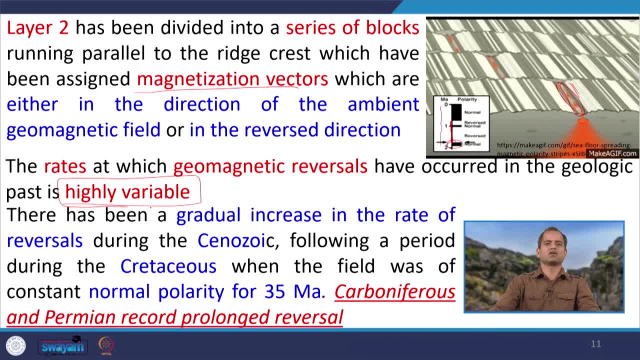 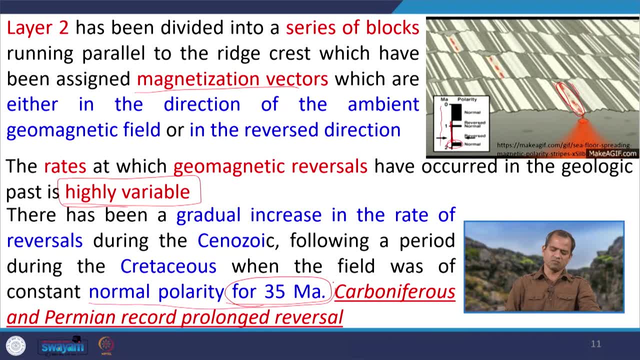 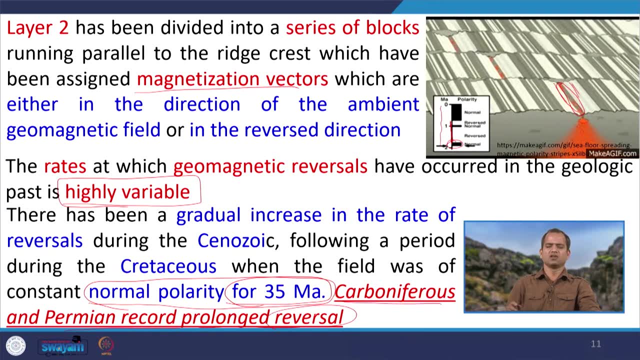 of during Cretaceous, when the field was constant, normal polarity, about 35 million years. So the Cretaceous it was recording maximum normality and Carboniferous and Permian it is record prolonged reversal. So Carboniferous, Permian it is highly reversal period, the duration was reversal period and 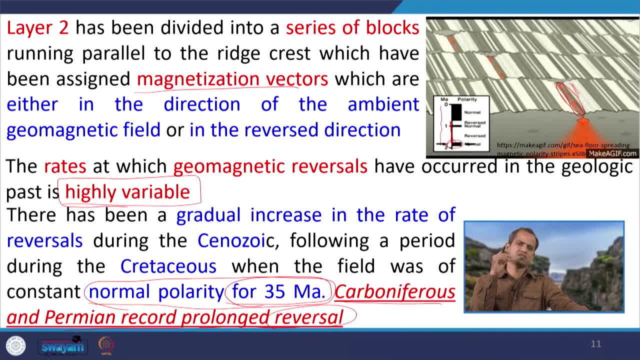 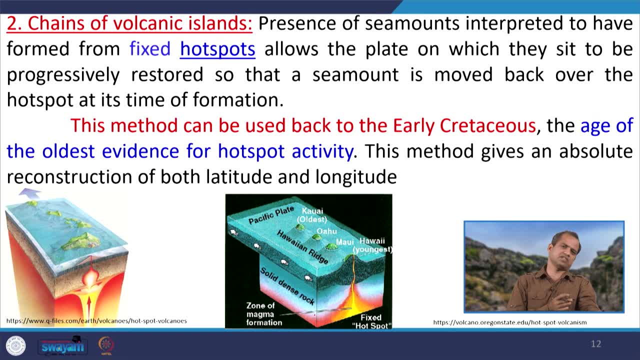 this Cretaceous period. it was recording this high time. it is normal period Now. this is one evolution Evidence that, yes, seafloor is spreading. so that is why we have a magnetic strips and that is recording the normal and reverse magnetization. Another is the chain of volcanic island that we have already discussed during this continental 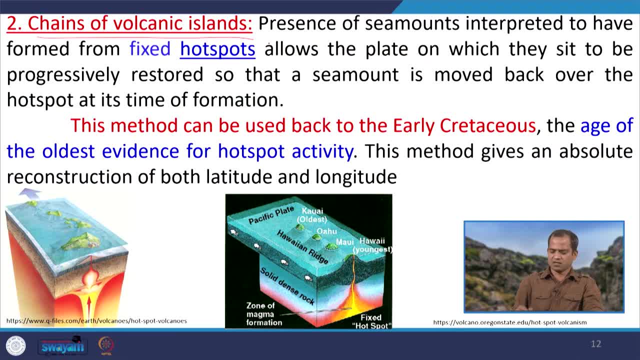 drift when we are talking about this chain of volcanic island. if you see, we have a volcanic system, that is, this hotspots, and this plate is moving. we have different hotspot, islands are there and this side is the older, this side is the younger and we can calculate the. 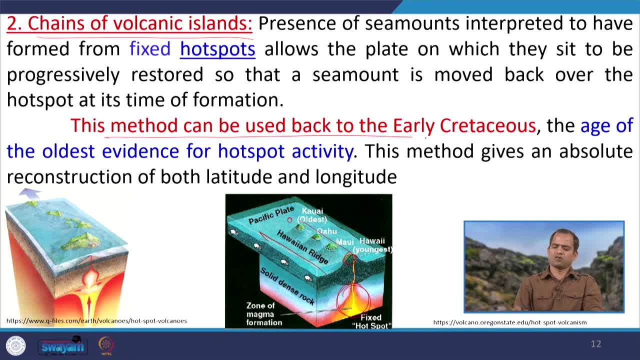 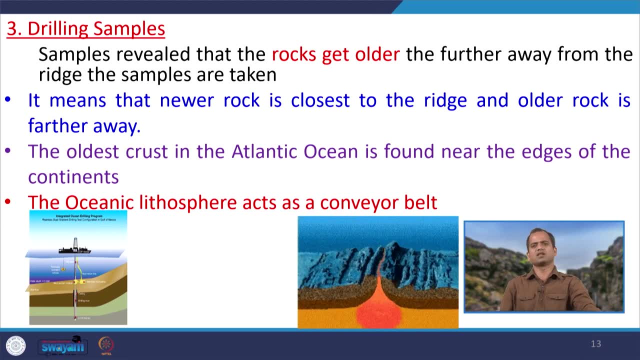 rate of movement from here, and this method can only used up to early Cretaceous, because beyond that this earth crust has already been destroyed. Then third is the drilling samples. we have deep marine drilling projects. So during drilling project, if you are going away from this side, that means away from the 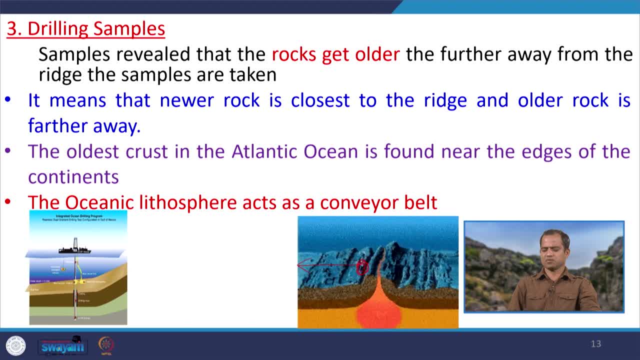 mid ocean ridge. we are drilling a system here and we are drilling a rock here and we are taking the rock, We are dating it and finally we will get. we are getting the older side of rock here and we are getting younger side of this rock here. 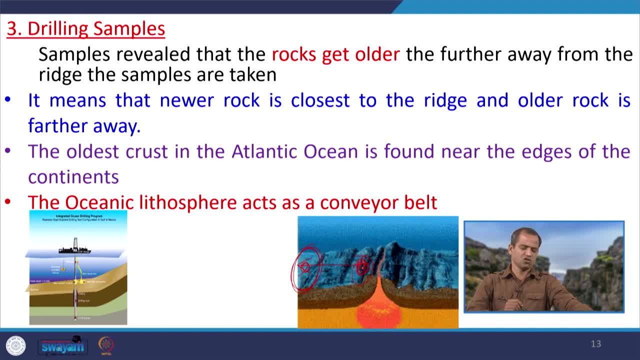 So that means younger rocks near to the mid oceanic ridge, older rock away from the mid oceanic ridge and the oldest part of this live ocean floor. we can get near to the trench of that basin. So here, if you are going to this marina trench in the Pacific, you will find the oldest oceanic.